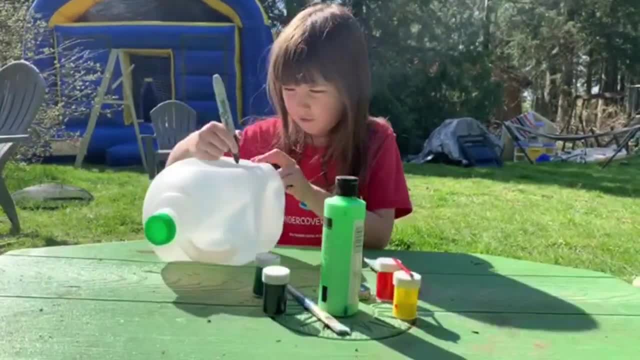 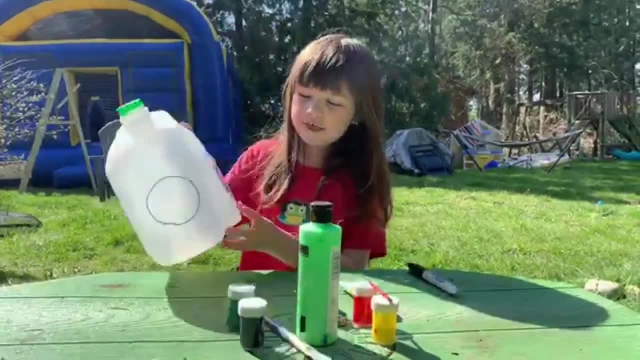 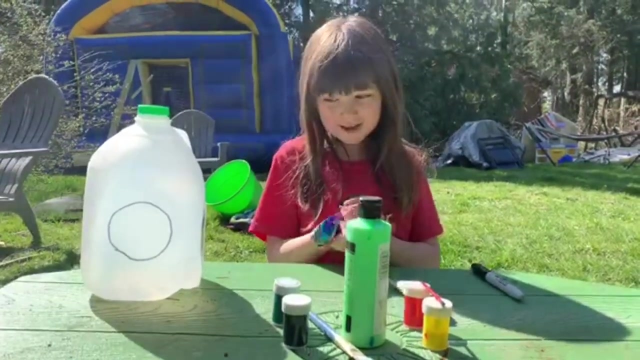 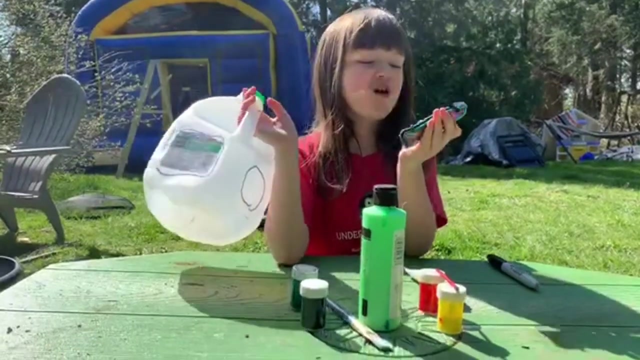 So this is how it turned out And the next step. you might need one of these. Actually, you will need a grown-up to do this part, unless you're already a grown-up doing this project. So you will take a knife. 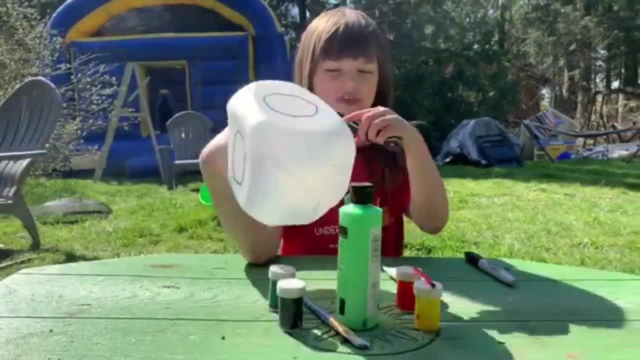 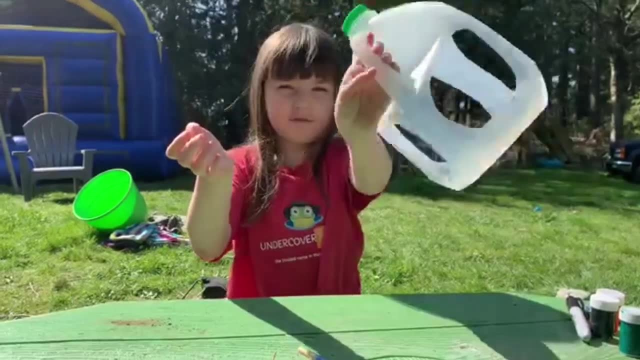 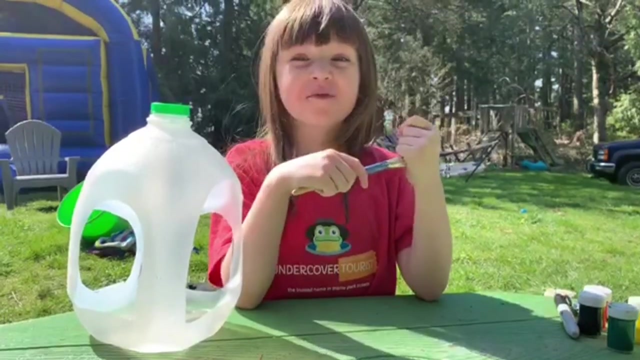 You will use a knife And you will cut around all of these circles, all of the four circles. So right now we have cut all four sides out, as you can see. Don't forget to subscribe, hit that notification bell and give a big thumbs up. 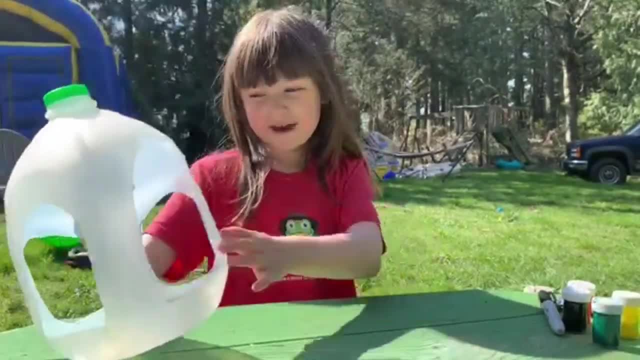 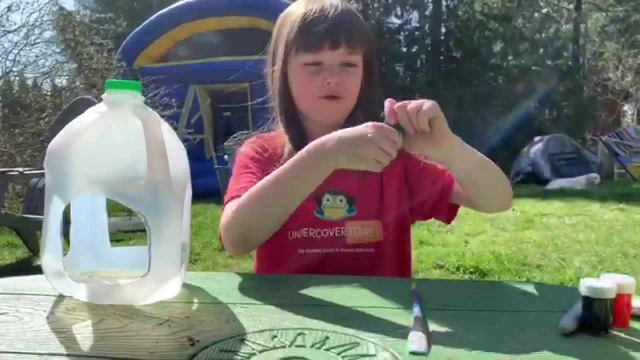 Right now we're going to paint it. It's going to be kind of hard to paint because my mom messed up, So, yeah, we can just start there and move on. I'm going to rip open this paint. Don't actually rip it, because then you'll get very painted. 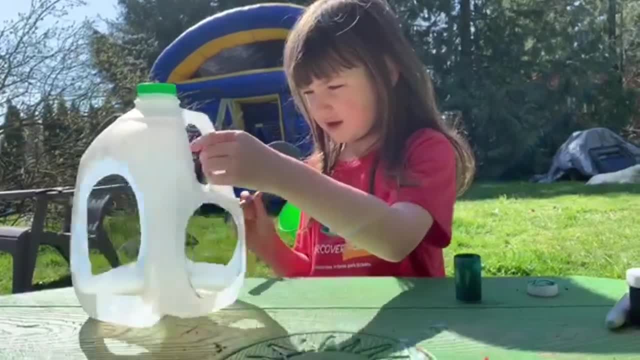 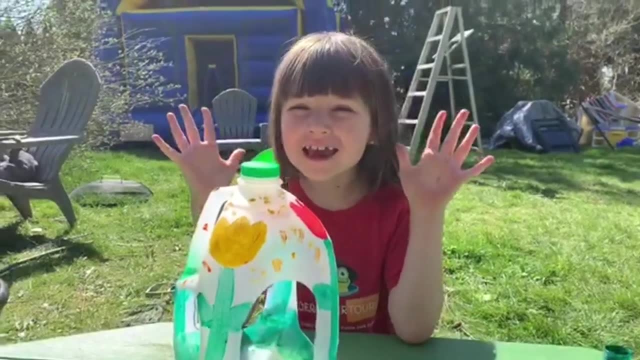 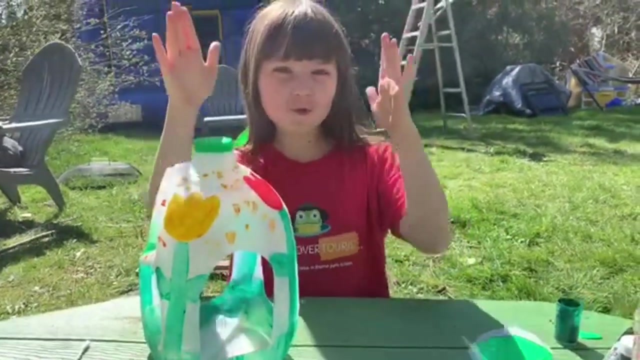 That's quite a lot of grease I got. I'm going to do it like this. There we go. So we painted it And right now we're going to be doing, doing, doing, doing. Just going to tell you what we really did. 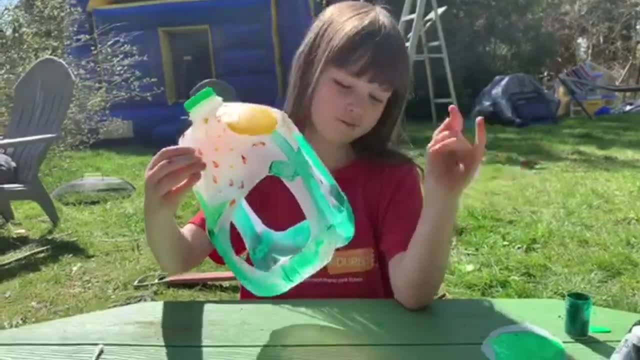 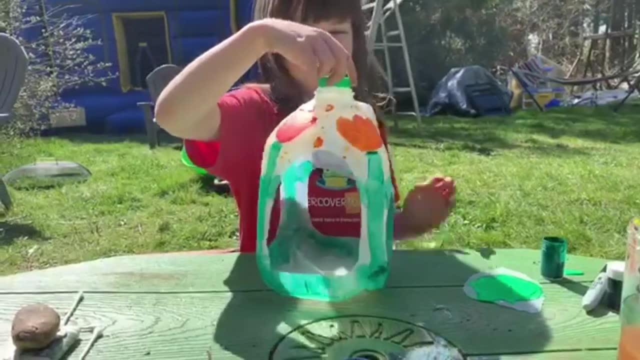 So we did it with some tulips, and then we had some dots, Then we put some grass on, Just to do the extra touch. Actually, yeah, we do need to poke some holes in the top, Or you can just hang it from here. 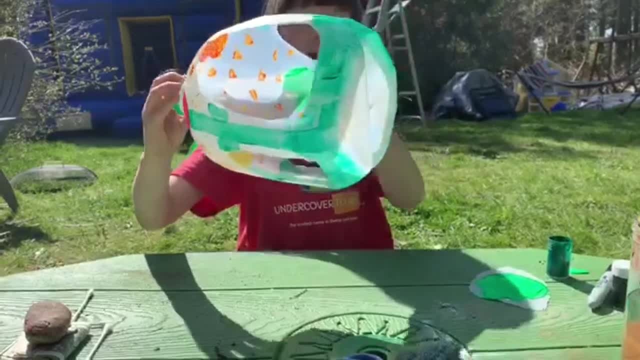 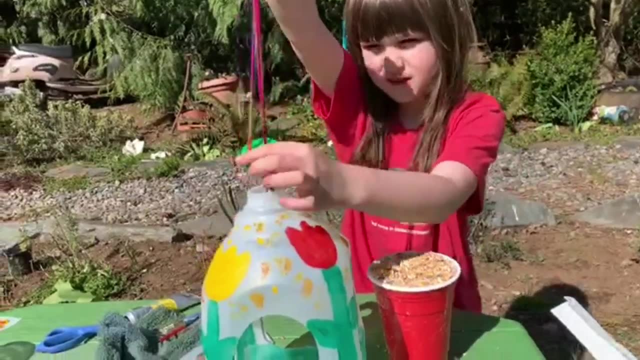 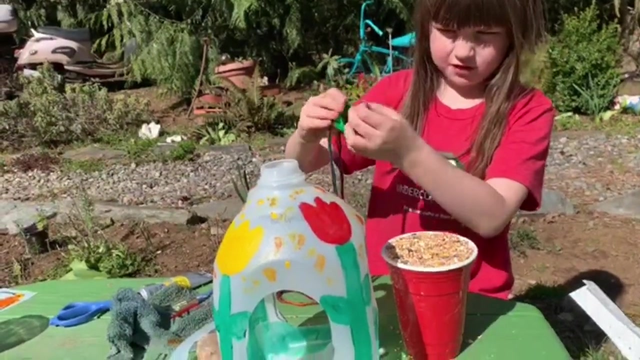 Yeah, But then the birds will fall out, So yeah, So if you were wondering how we're going to put that on there, we have some string and we're tying it under, But if you want to, you can take off that excess part. 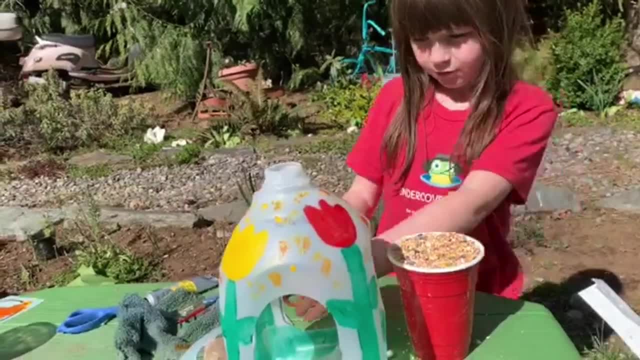 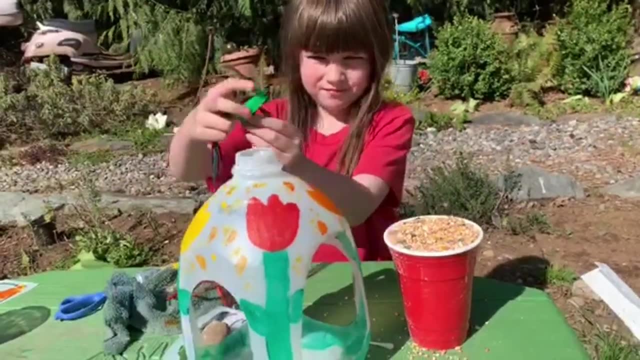 But I don't think we need to Plus. the birds will just focus on the bottom part with the food. So I'm going to screw it on just like a regular milk cap. It would be squirty. It would be screwed on just with the strings inside.